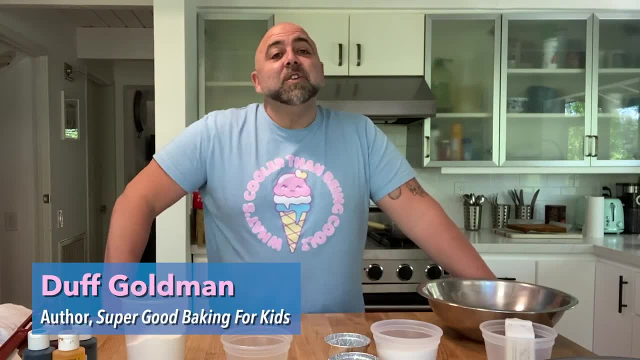 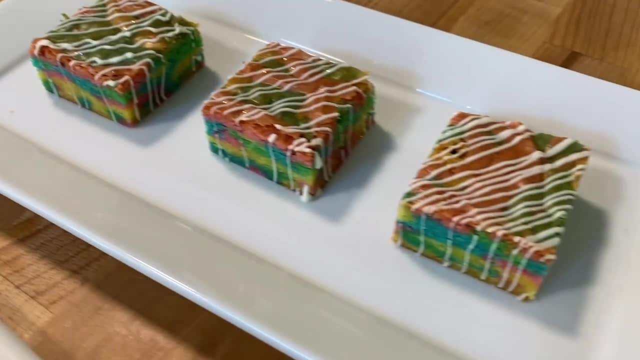 Hey, what's up guys? So I just wrote a new book. It's called Super Good Baking for Kids. It's not just for kids, though. It's got a ton of super cool recipes in there. One of my favorite recipes from the book is rainbow unicorn brownies. I was in Oklahoma and I was talking to this little kid. 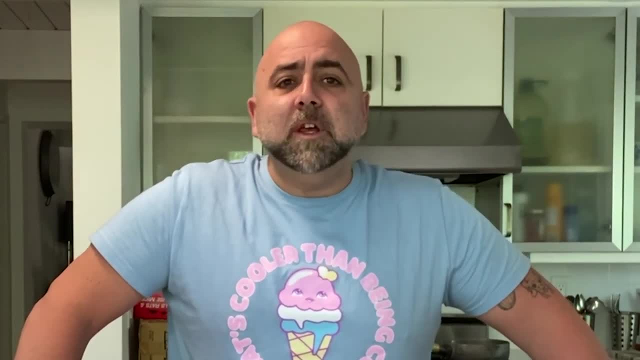 and I was like: hey, if you could have any recipe like in a kid's baking book, like what would you want? And she was like: I want rainbow brownies. And I was like: brownies are brown, right You? 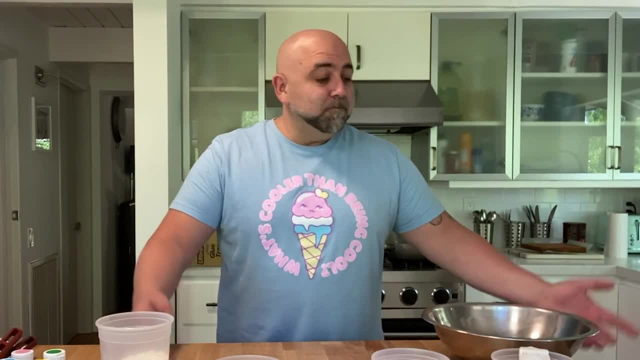 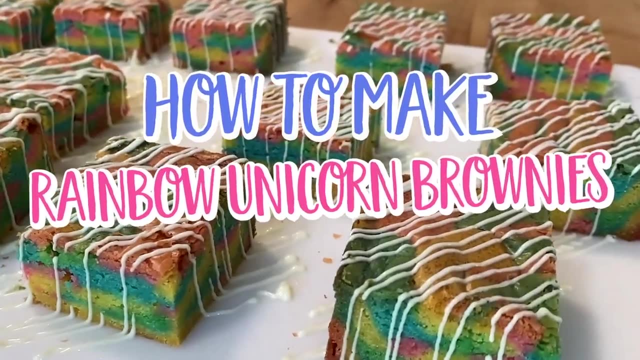 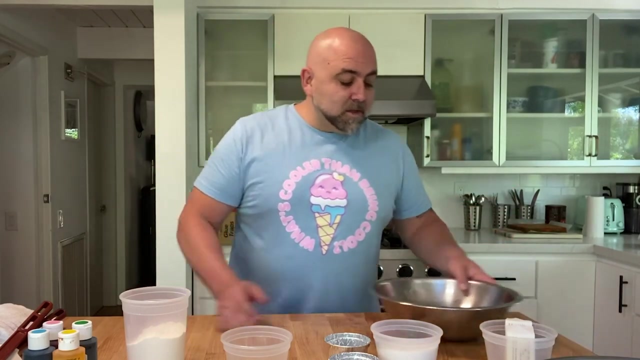 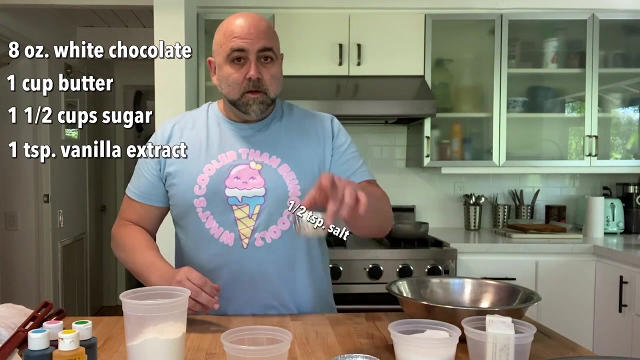 can't make rainbow brownies, She's like: well, that's what I want, So figure it out. So I figured it out and I'm going to show you guys how to make it All right. So what you need is some white chocolate, butter, sugar, vanilla, salt- always important, Never forget the salt. 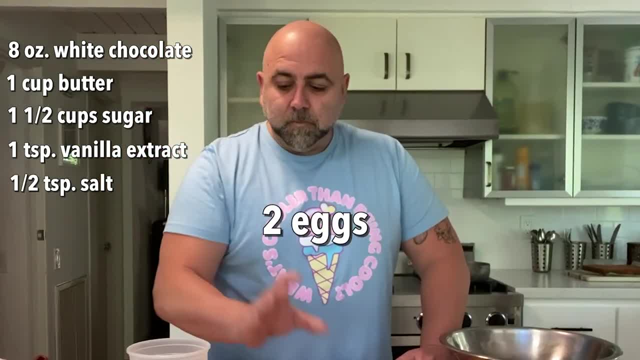 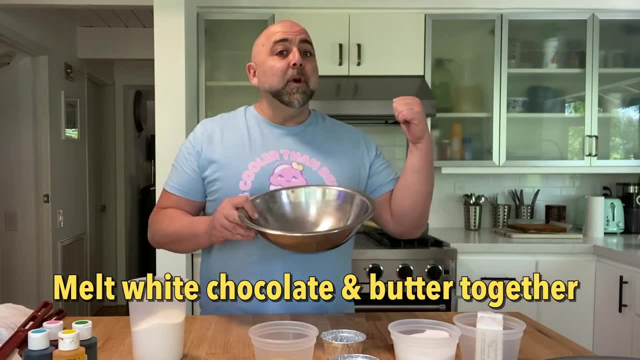 Everything sweet has a little salt in it. Everything, Two eggs, flour, That's it, All right. So the first thing we're going to do is we're going to make a little bit of a is we're going to melt this chocolate with the butter on the on a double boiler, because I don't. 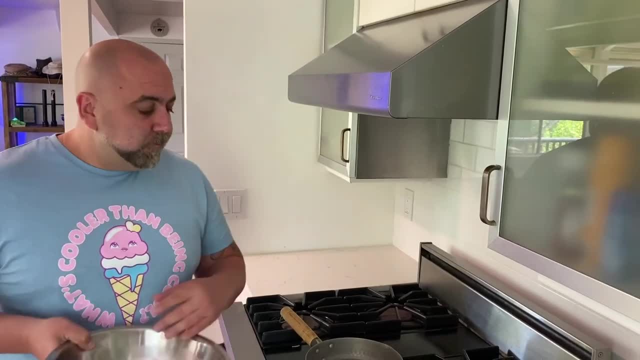 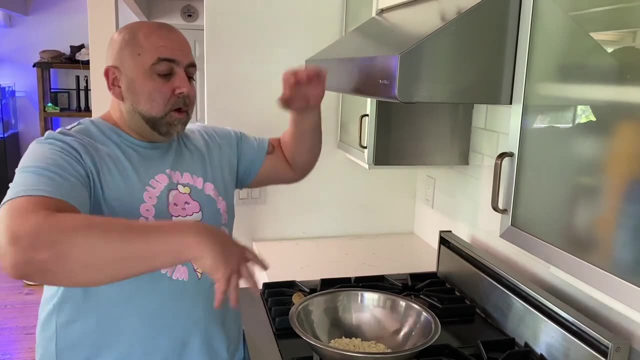 trust microwaves, All right. So here's the thing: I have chocolate in a metal bowl and I have hot water that's simmering. It's not boiling. You don't need it to be like a super crazy, you know. 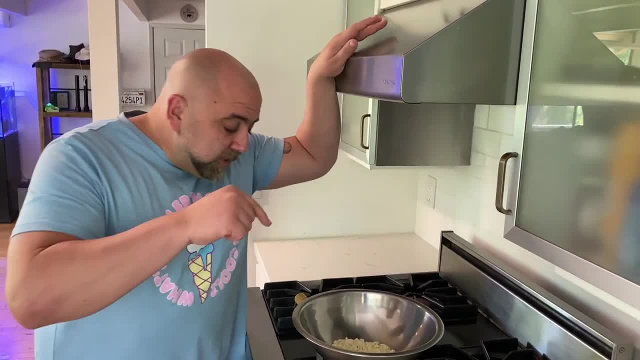 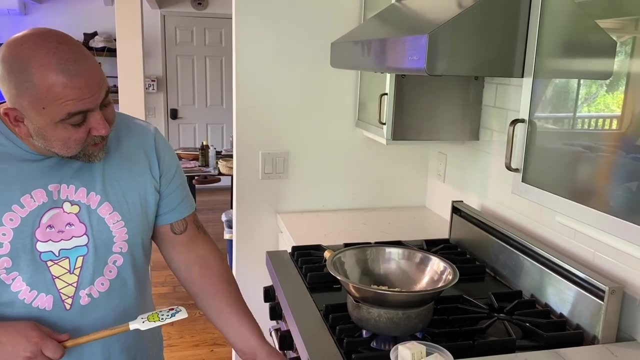 all the steam coming out, because if too much steam comes out, what will happen is the steam will get in there and the chocolate will seize. The other thing you want to watch out for is, if the heat is too high, the fire goes up around the pot. 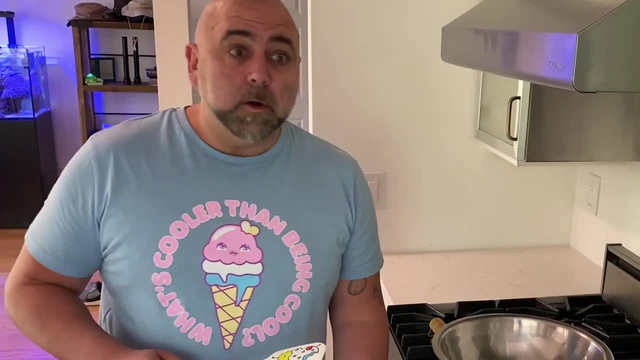 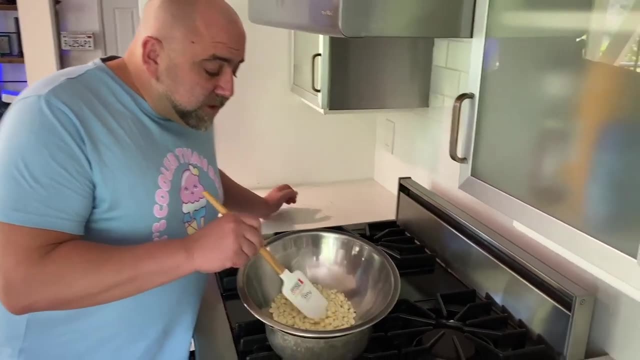 It's hitting the bowl And if that happens the chocolate will burn. So low heat. get it up to a boil and then turn it on low heat. You stick it on here and you'll see it's already almost melted. When you're doing this, make sure you always have a towel so you can grab the bowl. 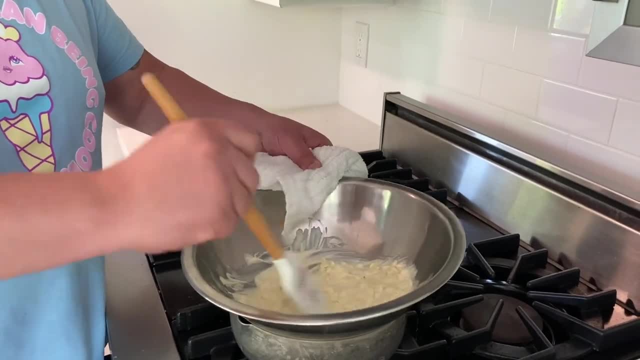 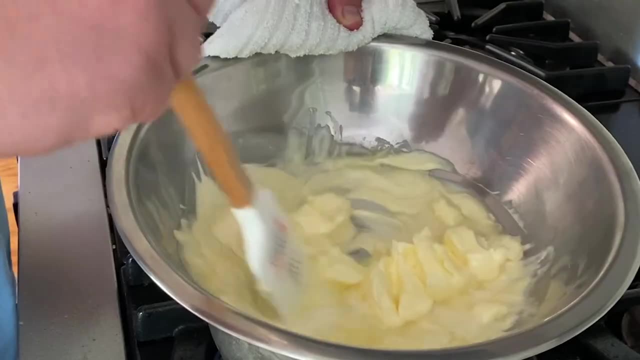 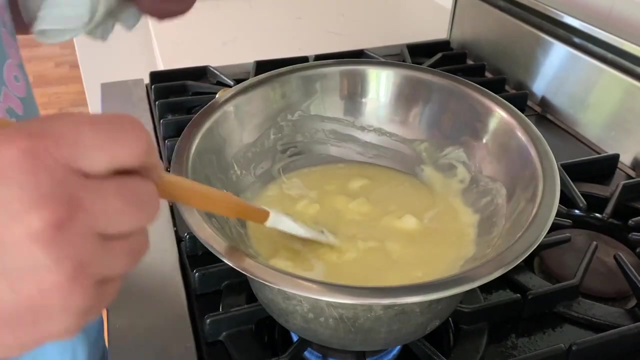 It's already almost melted. So now what I'm going to do is add the butter. So give it a poke, stir this up and just gently stir it. You don't want to like go too fast because you're trying to get the chocolate and the butter to like really mix well together. 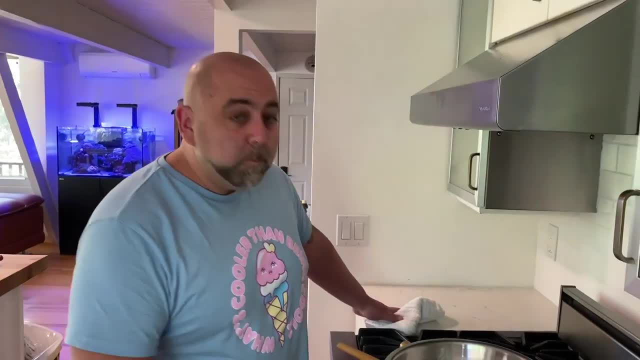 There we go Now. the residual heat, the rest of the heat that's in there, will melt the rest of those mums. You can see it's not going to like totally combine. That's okay, Don't worry about it. Add the salt. 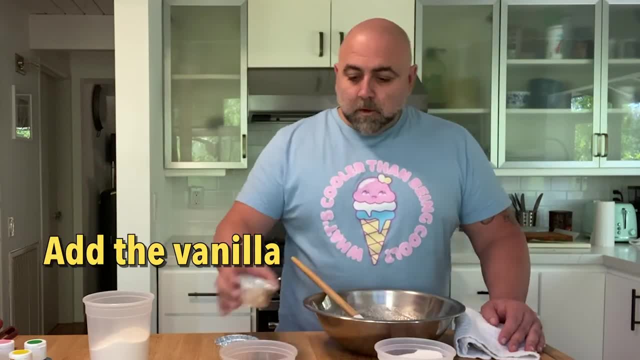 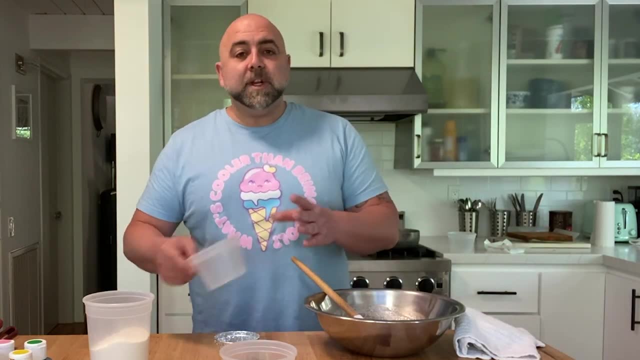 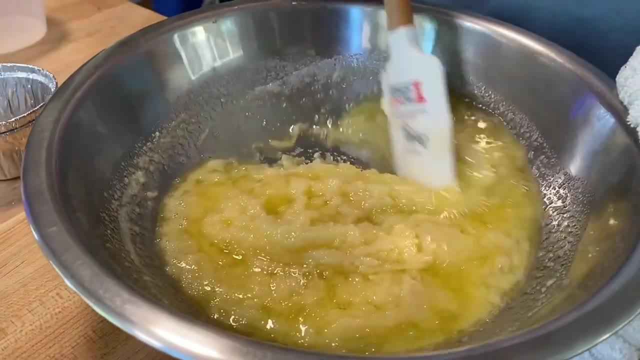 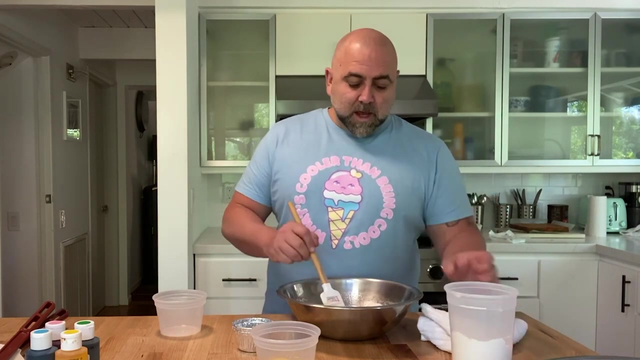 Very important- Vanilla and the sugar. Okay, What that's going to do is it's going to start bringing the temperature down and bringing this together, So we're stirring this around. You can see it still doesn't look all that great. Right, That's okay. I'm going to start with the flour. I'm going to put in about like a third to a half of that. 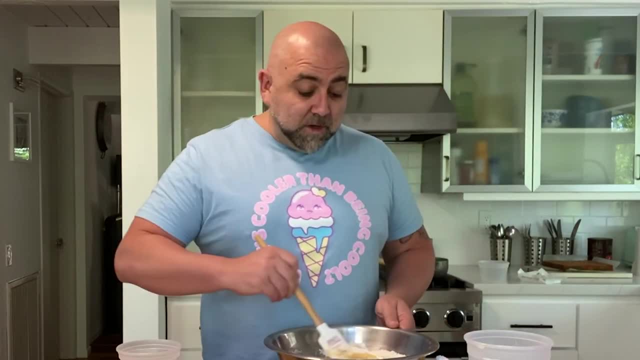 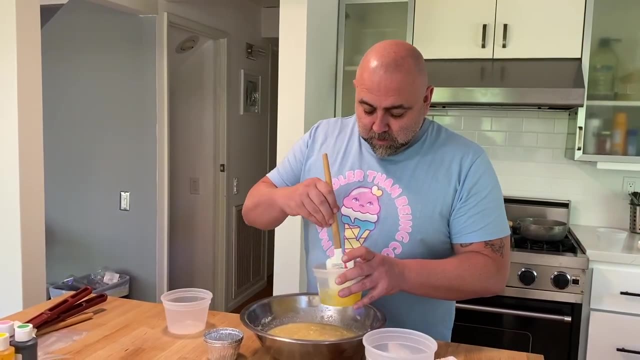 All that starch in the flour is going to make the chocolate and the butter combine. Okay, Now we can do the eggs. I just want to pop the yolks to make sure that they get mixed up in there. real good, Now I'll put the rest in there. 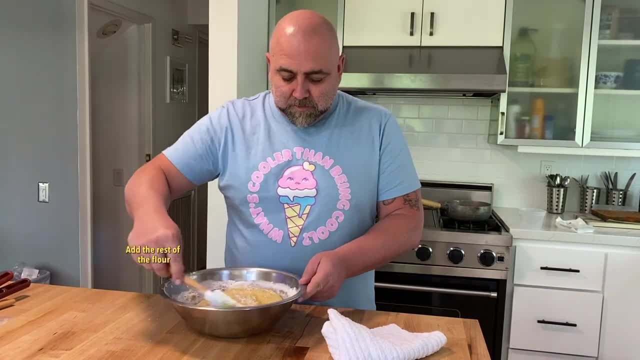 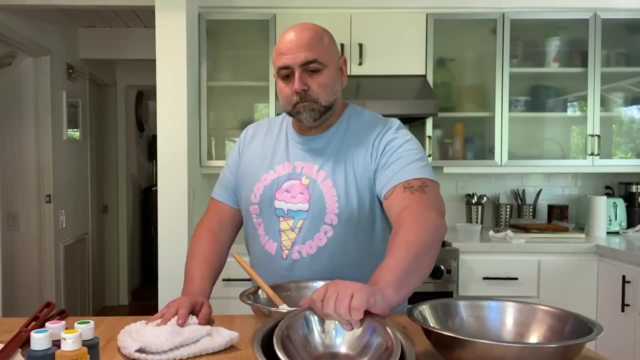 Okay, Make sure you get all that flour off the sides. here And there you have it. There's brownie batter. Now I'm going to take some bowls. This is the fun part. I'm going to put a little brownie batter in each bowl. 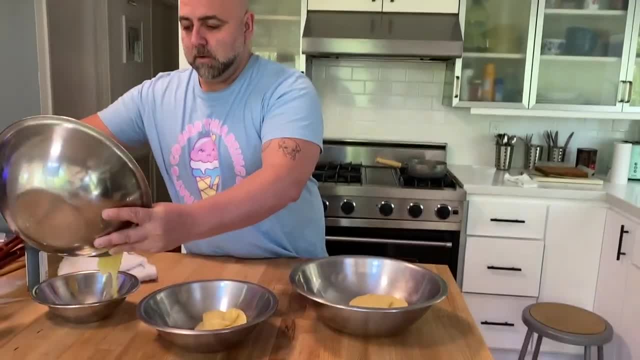 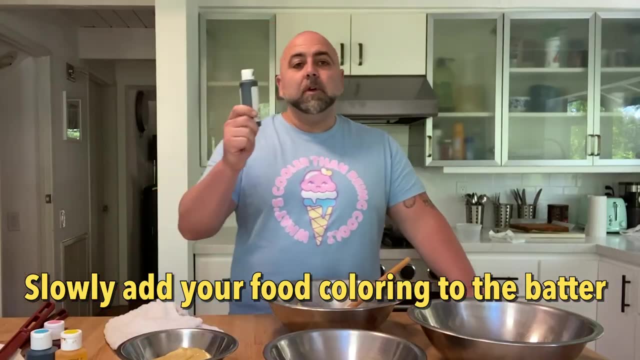 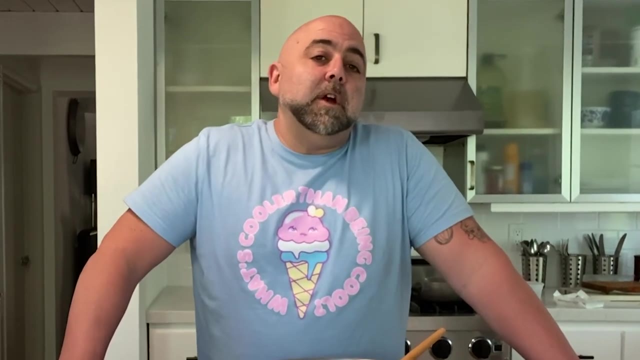 All right, Try to divide it roughly, equally, Okay, And then I'm going to put a little drop of green. Now here's the thing with food coloring. My food coloring is for super famous professional TV star cake decorators, And it's really strong. 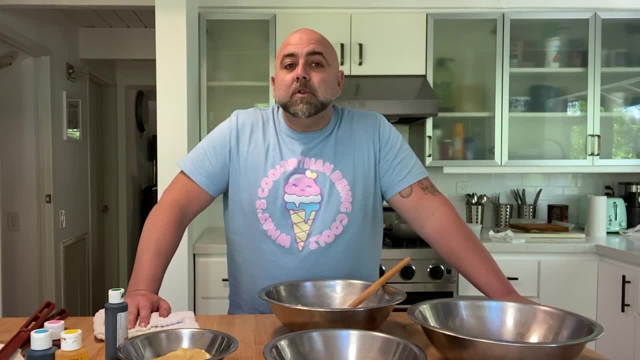 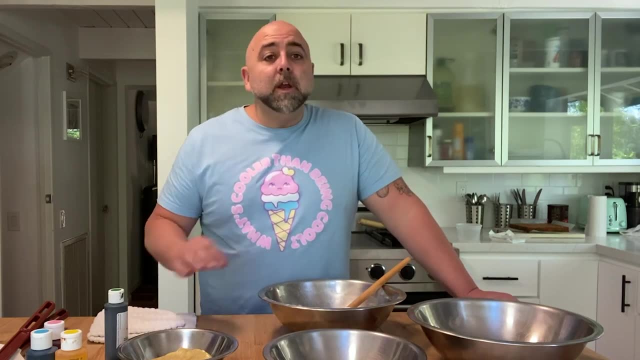 The food coloring that you're probably using. you got at a grocery store. That stuff is a lot thinner than this, So you might need like two drops or three drops. I only need one, But if you are using the gel, a little goes a long way, especially pink. 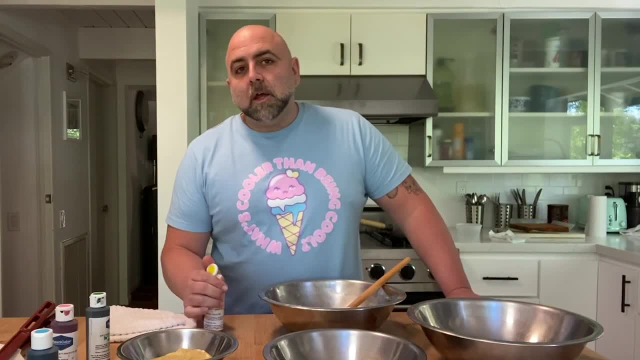 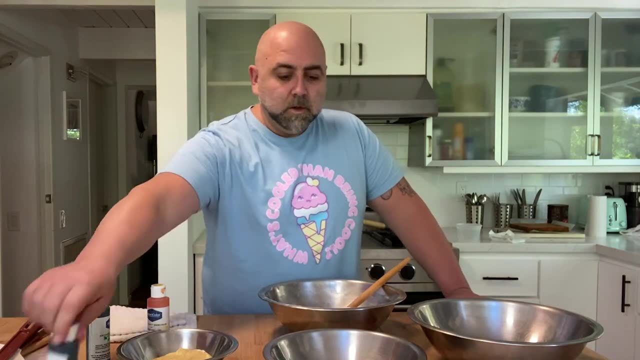 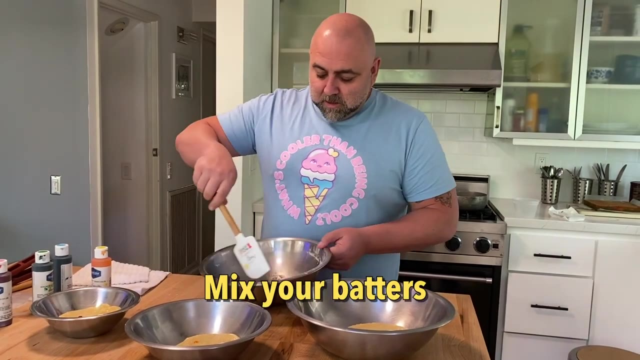 Little dab will do you Yellow, And it's already yellow. It's more of just like a you know weird cake batter color, So that yellow is going to give it, you know, a little brightness. Then blue: Same thing, Just a tad. Just a little bit. That's all you need. All right, Let's mix. 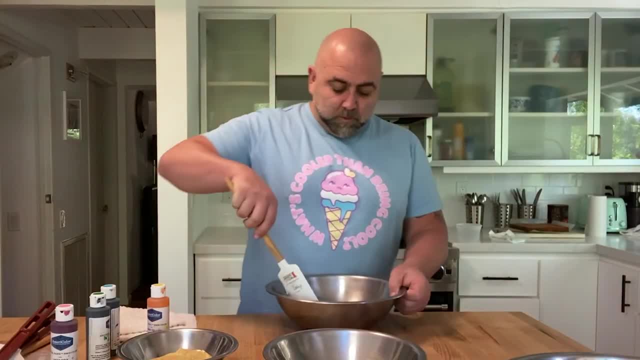 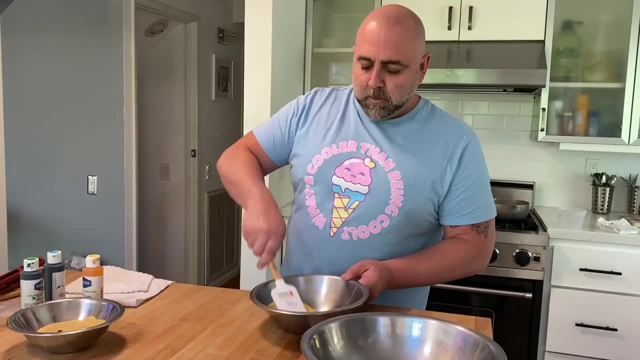 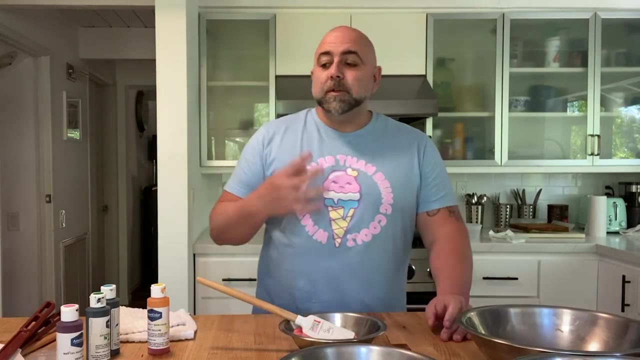 Yeah, that looks good, All right. There's the green. Let's do the blue, Okay. Yellow, All right. Pink, All right. So now we have four colors. I'm going to take four piping bags. If you don't have piping bags, you can do this with spoons. 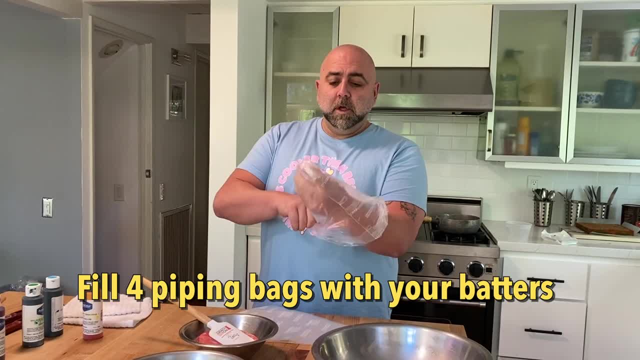 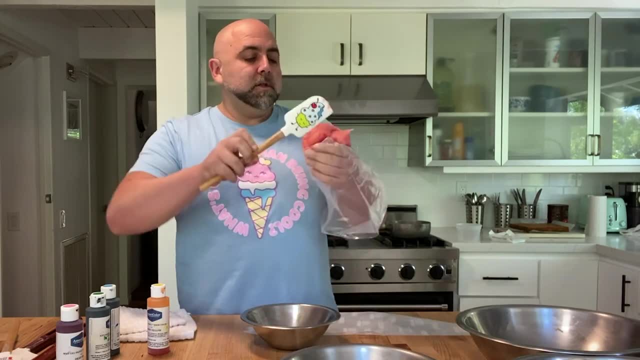 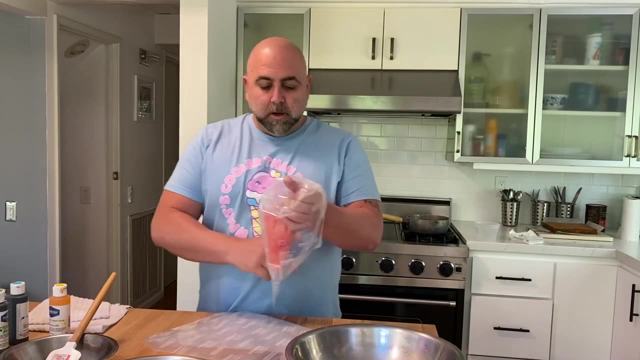 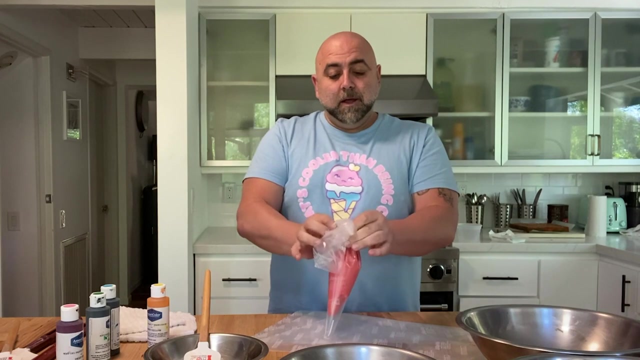 So the piping bag we're going to do- I want to get it open really really far- Pick up all this batter, Stick it into the piping bag, Just like that, All right, And then, if I have the room, what I like to do is tie the back of the piping bag So that 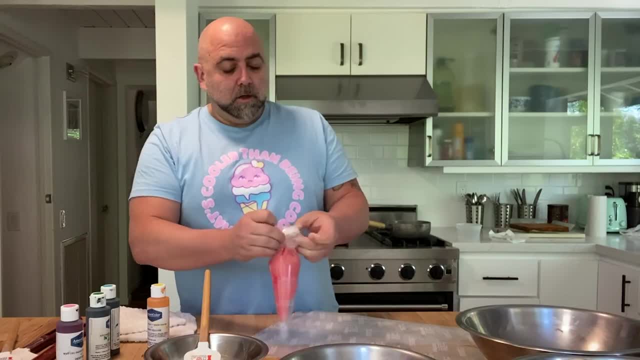 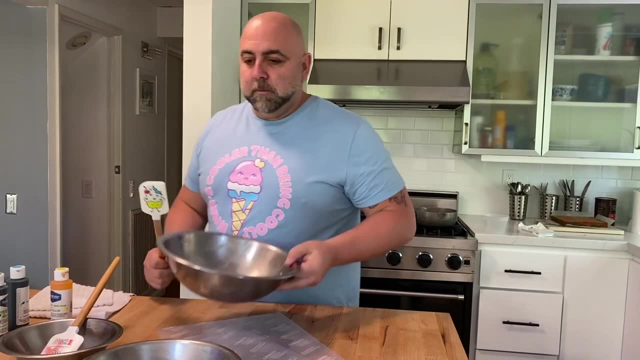 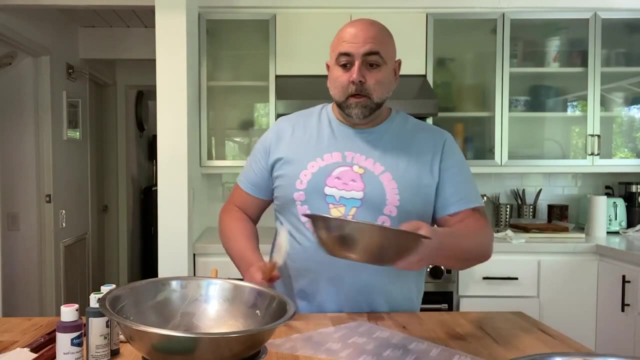 way when I squeeze it it doesn't shoot out the back and go all over my hand. Blue, Look All right, Mr Yellow, Okay, Green, All right. So what I have here is an eight by eight square cake pan. 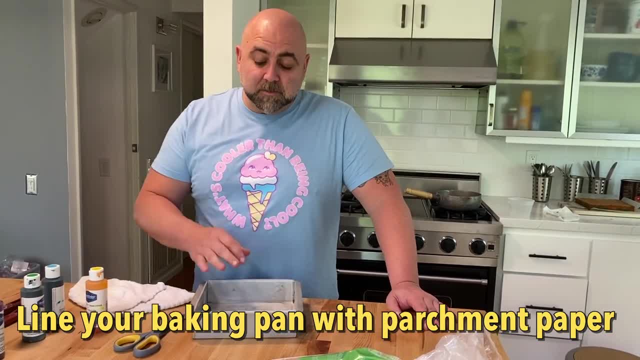 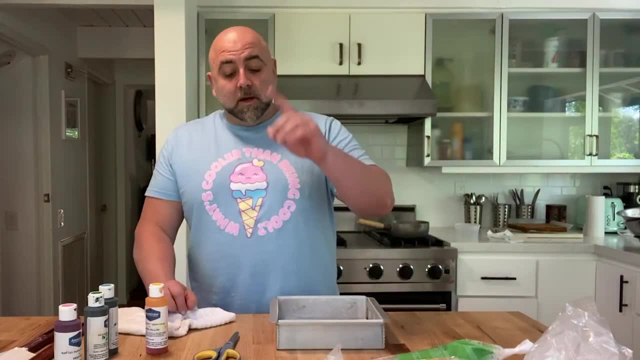 So I have two 12 inch by eight inch pieces of paper, And what that did was it created a little aside on each one and the pan's all covered, And then, when it's time to get this out, it'll be really easy. I just grab the paper and pull the whole thing out. All right Now. 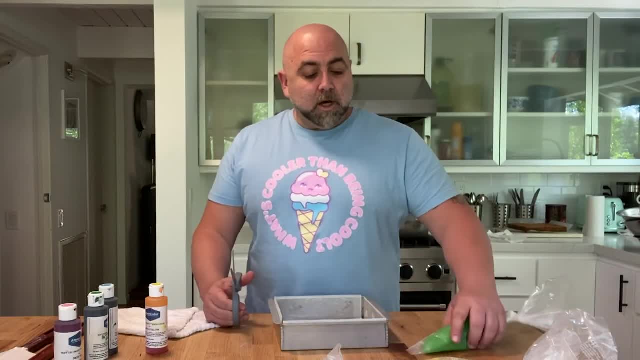 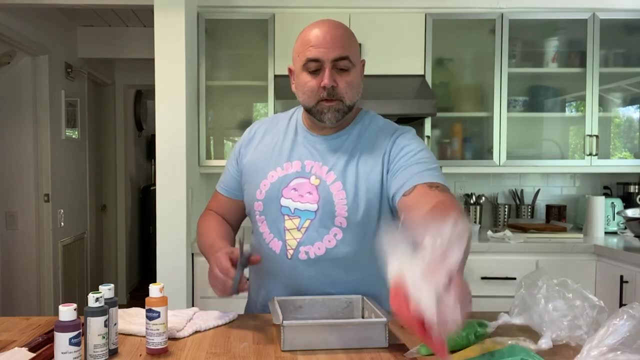 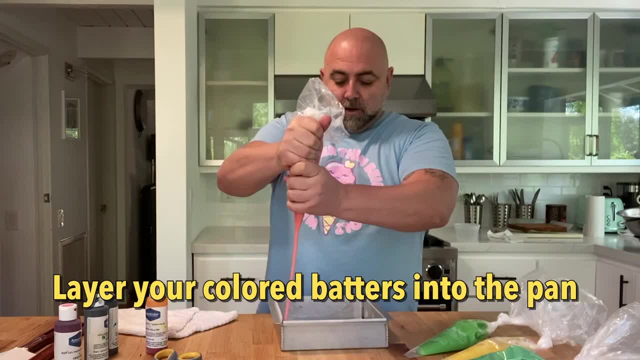 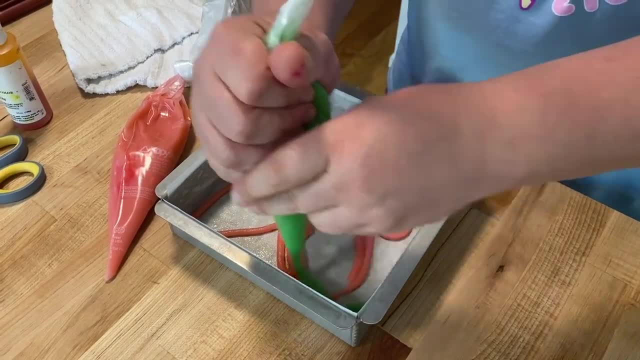 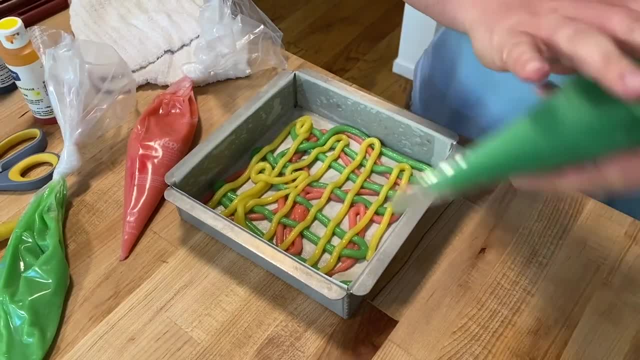 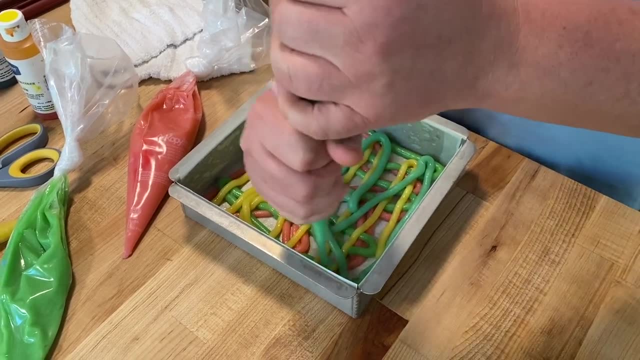 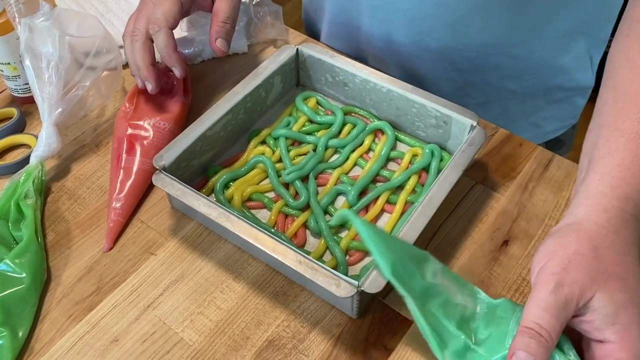 because every brownie has to have all the colors in it, Right? Ask any kid. Your kid will tell you: Better have all the colors in the brownie. So So squirt it in there. and then I'm going to go back to the first color, which was pink. 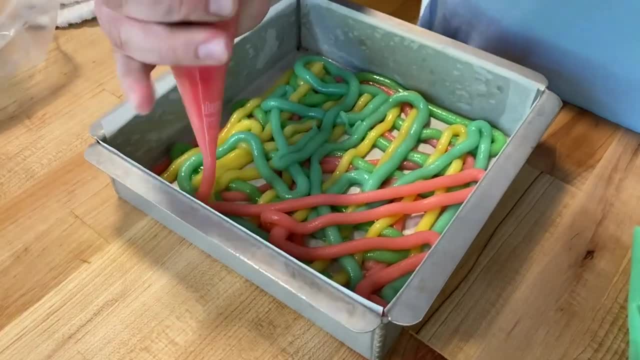 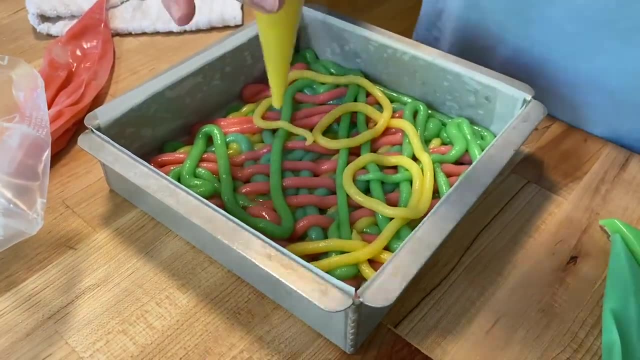 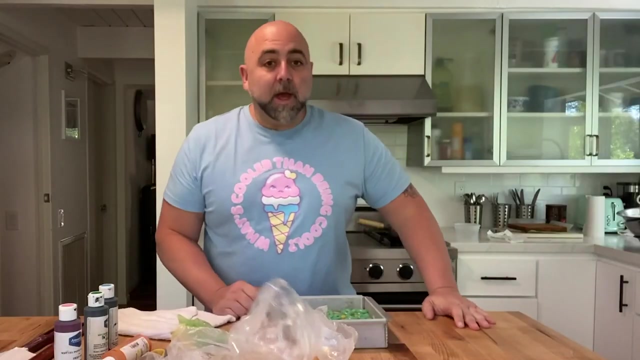 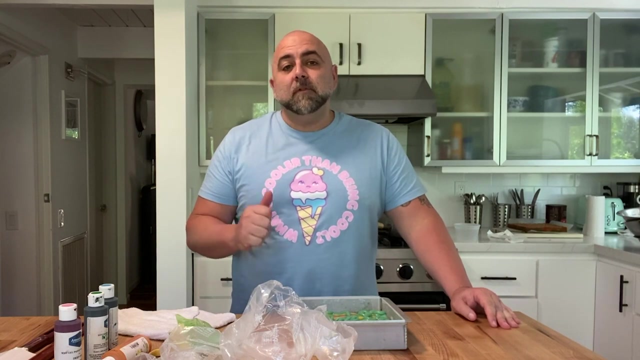 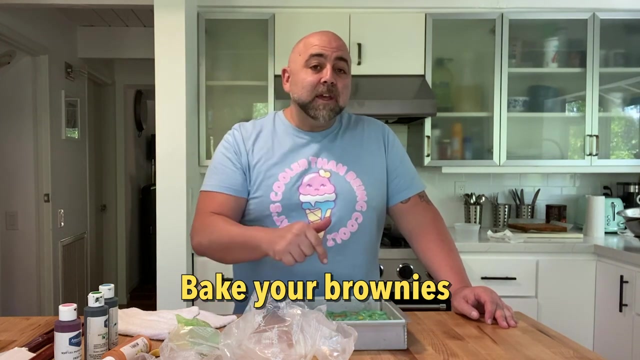 do another layer of that. Okay, there you go. Now. it looks super fun. So what we're going to do is we are going to bake this in the oven at 350 degrees for 40 to 45 minutes, and I will see you back here when they're done. 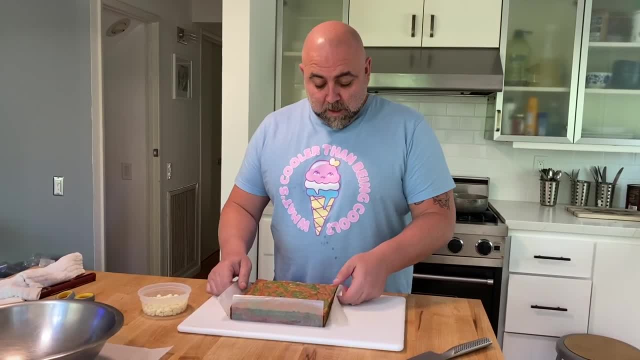 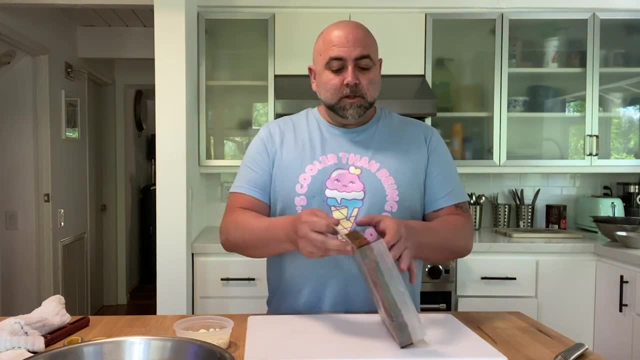 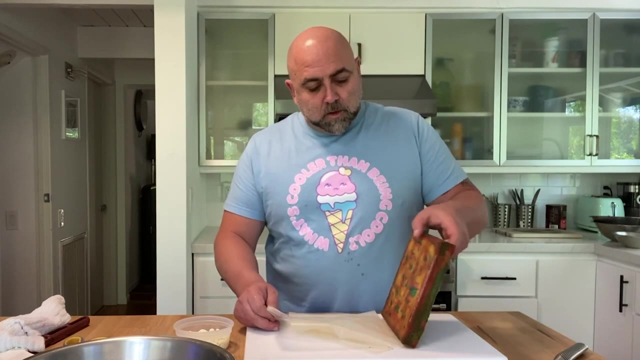 All right, here they are. And then, here I showed you the paper. that's how you get it out of the oven. Now these are nice and cool. Let these cool on a rack at room temperature for you know, an hour or so. 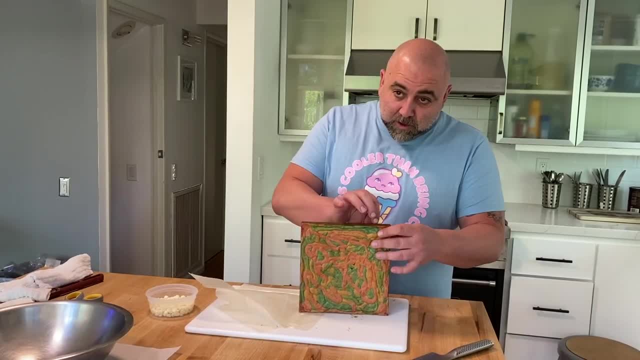 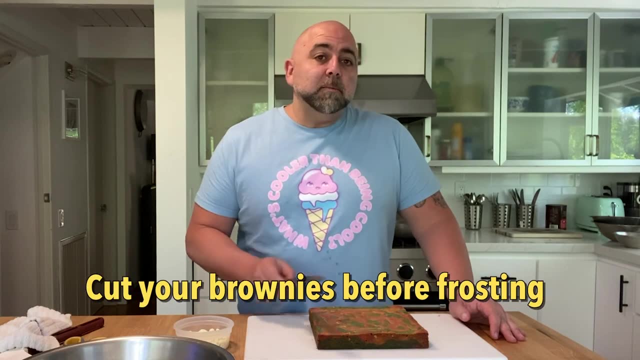 Okay, Just make sure they're nice and cool and then, when you pull the paper off, make sure you get all the paper. Sometimes there's little pieces that like to stick, All right. so what we're going to do now is cut them, because after this I'm going to 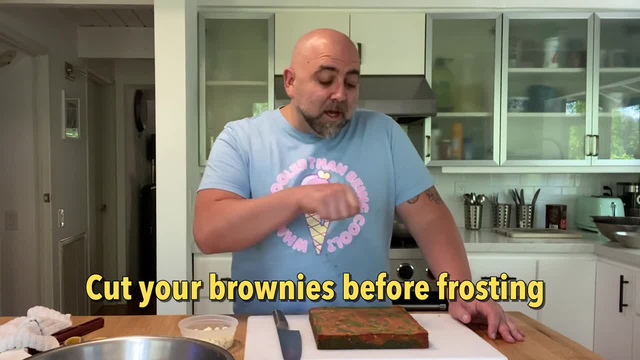 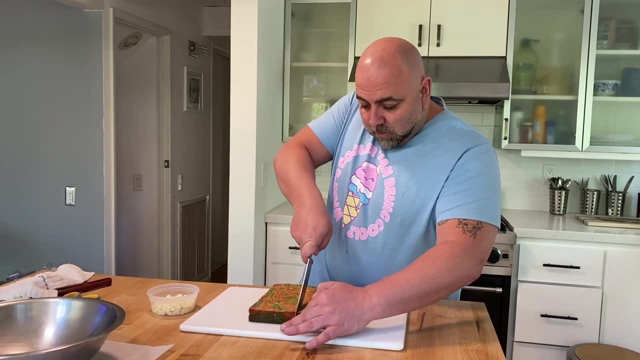 melt some white chocolate. I'm going to show you how to make a little tiny piping bag and then we're going to decorate the brownies. We want to decorate the brownies while the chocolate's still hot, So I'm going to go right down the middle here. try to go nice and straight. keep them even. 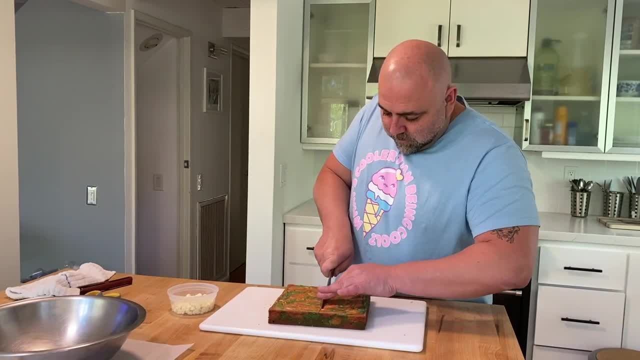 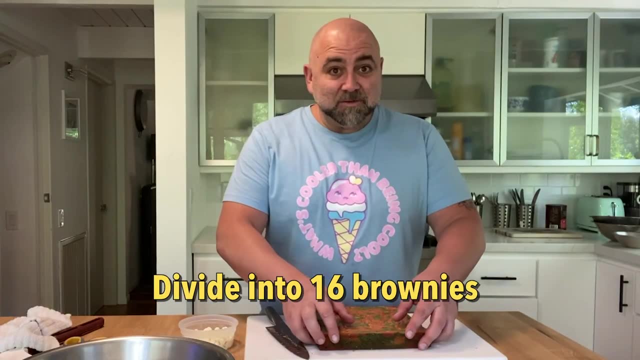 One, two, three, four. We got four brownies this way. four brownies, that's 16 brownies. You guys ready? This is the exciting part. Ooh, look inside, Look inside. Look how cool these look. 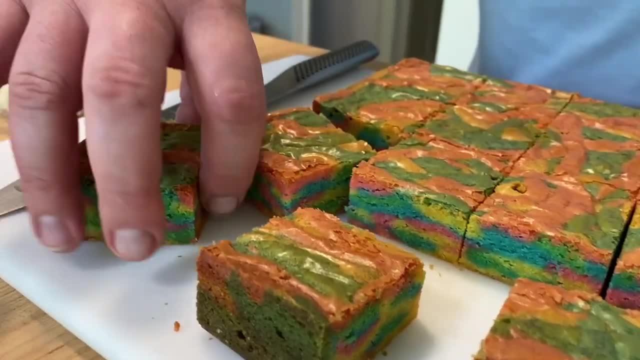 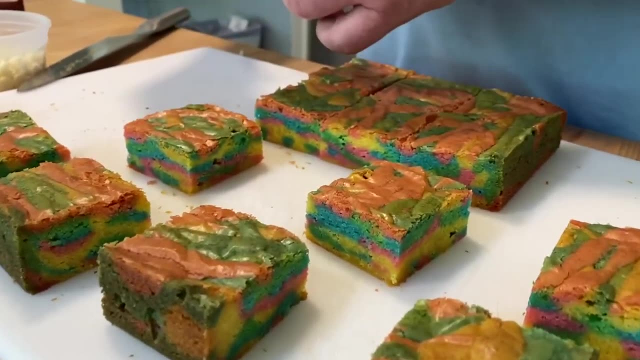 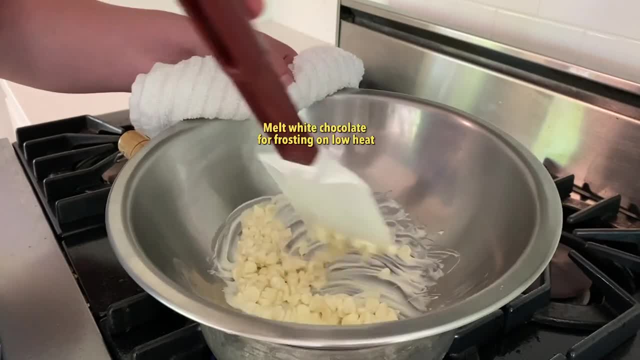 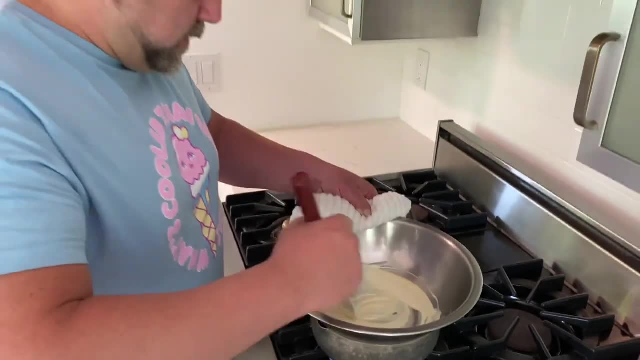 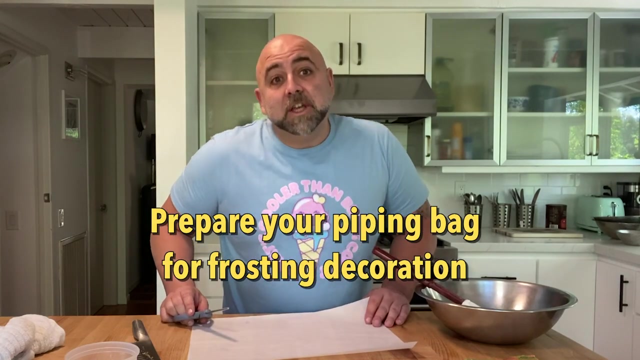 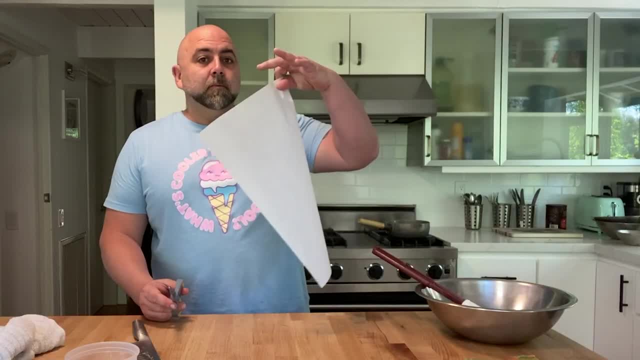 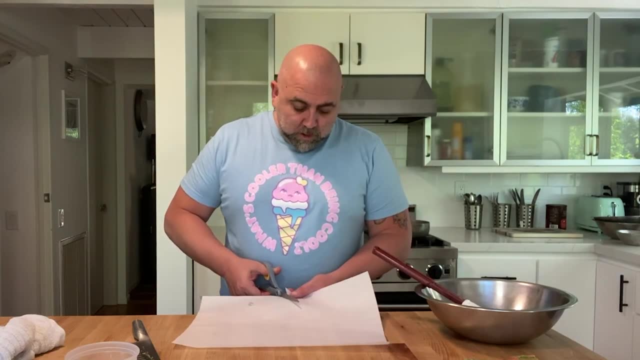 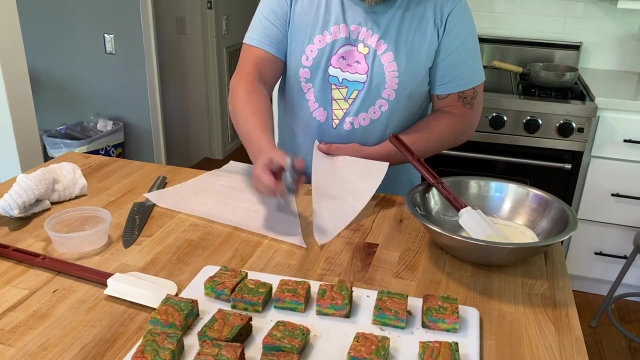 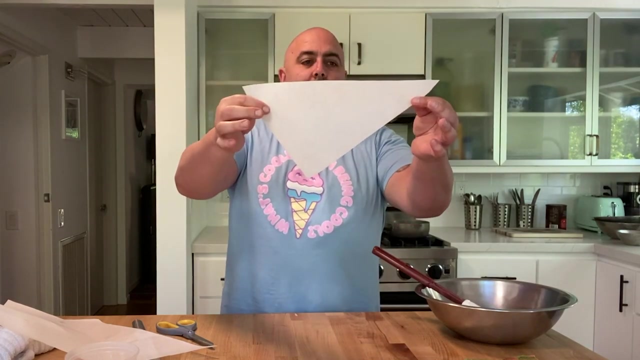 I have a piece of paper, Ordinary piece of paper. There's nothing up my sleeve. I'm going to take a pair of scissors and I'm going to cut a triangle, just like this. okay, Another triangle, a right triangle that is a little longer over here. 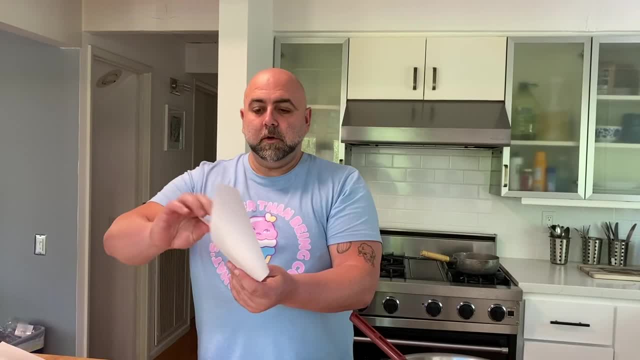 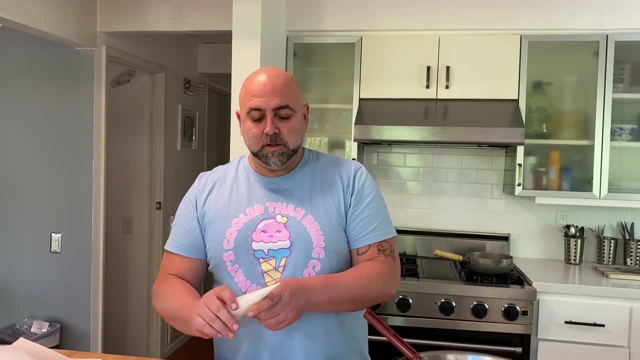 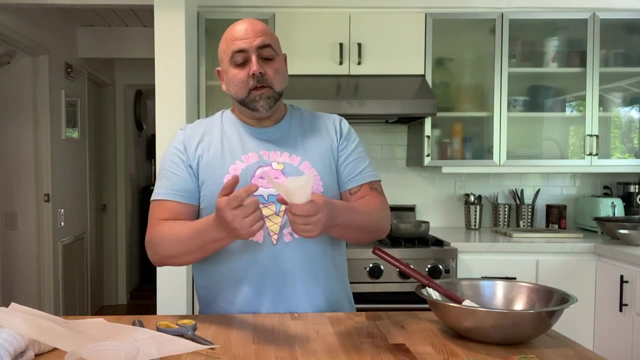 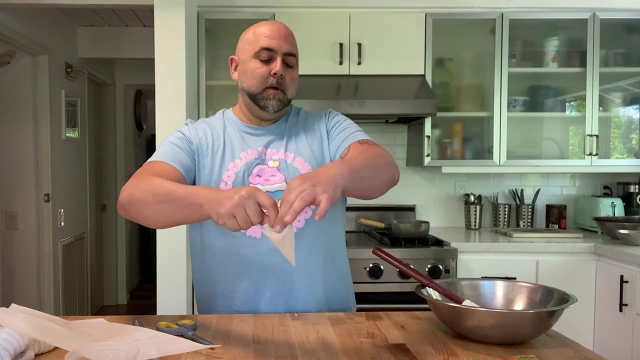 all right. So now what I'm going to do: fold it over and make a cone, And then take the long corner and wrap it around once, push the cone so the tip is nice and sharp, all right. And then you take the long corner here, fold it into there. Now you have a little tiny piping bag called 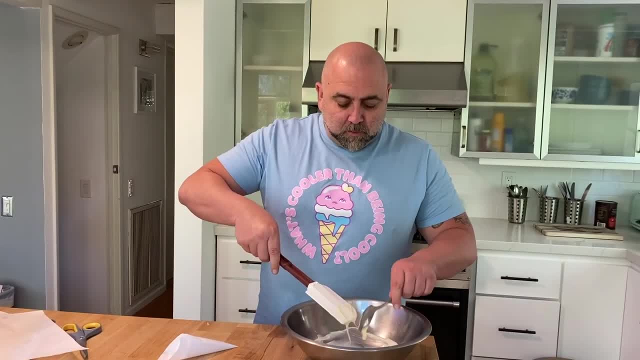 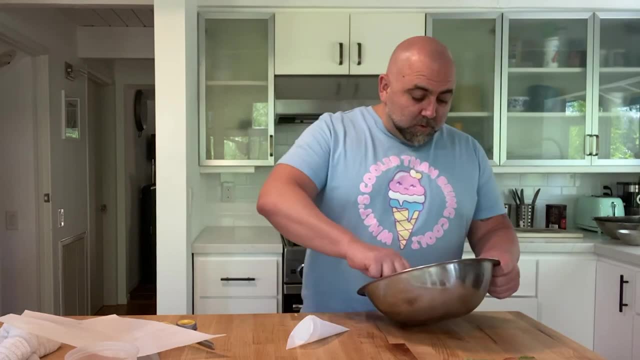 a cornet And I'm just going to take a little spoon, because it's easier to get the chocolate into the cornet with a spoon than it is this big old space And I'm just going to take a little spatula. So take the spoon, just get all this chocolate here and then you take your cornet. 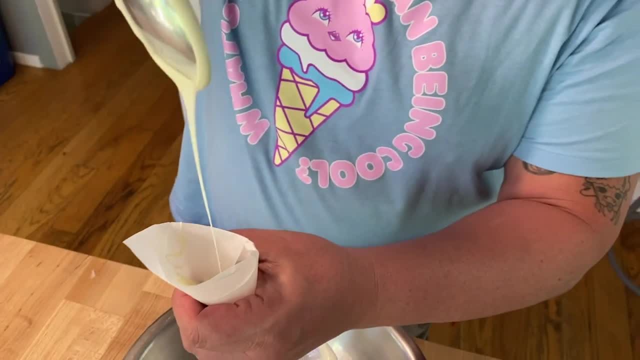 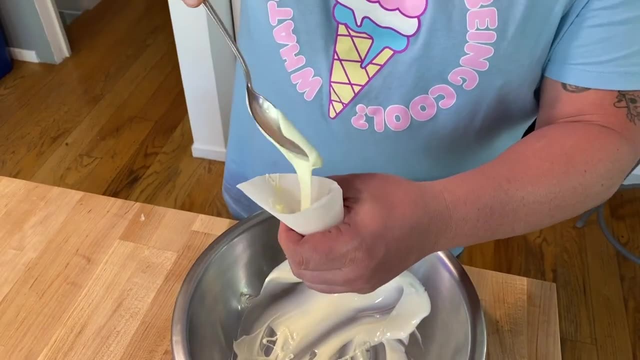 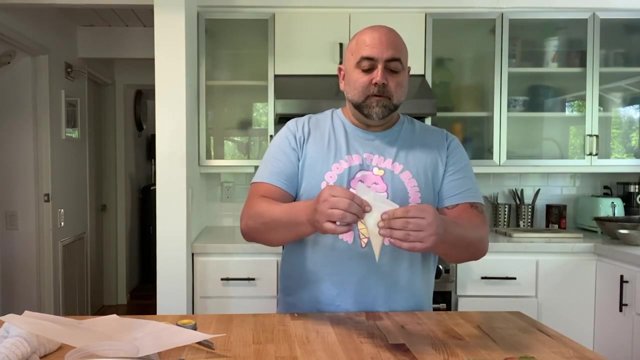 and just pour it in And try not to make a big mess, Try not to get it on your fingers or on the side of the paper. All right now. what I'm going to do is I'm going to flatten this out. I only 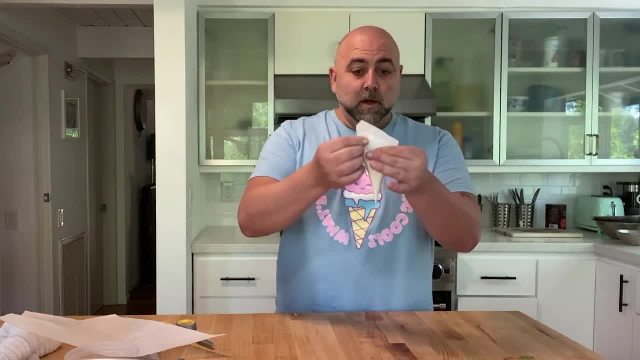 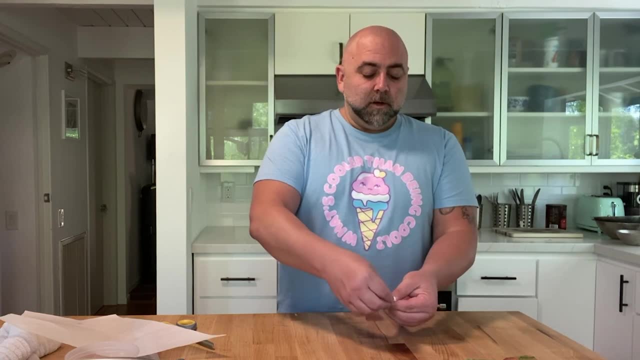 filled this about halfway because I'm not going to be able to fill it all the way through. So I want a lot of extra at the back here. So I'm going to fold it like this, And then I'm going to fold it like this And then fold. Now none of the chocolate is going to come out. Take the scissors. 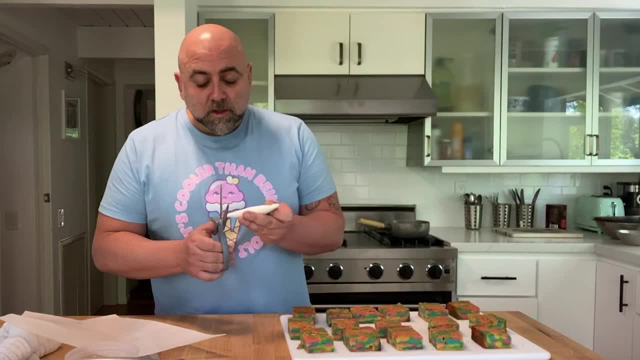 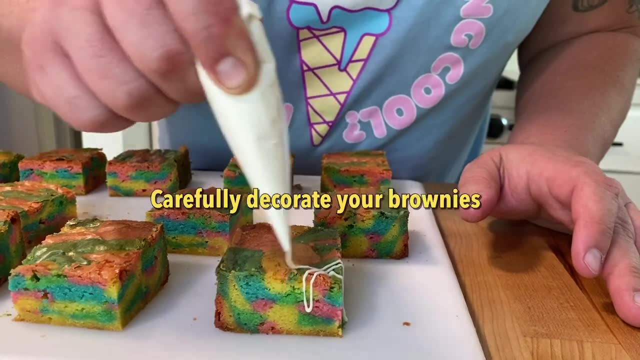 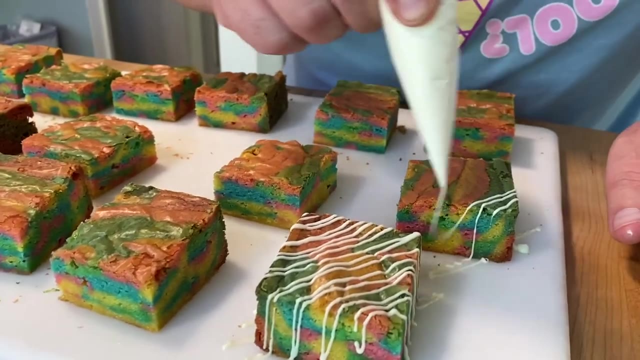 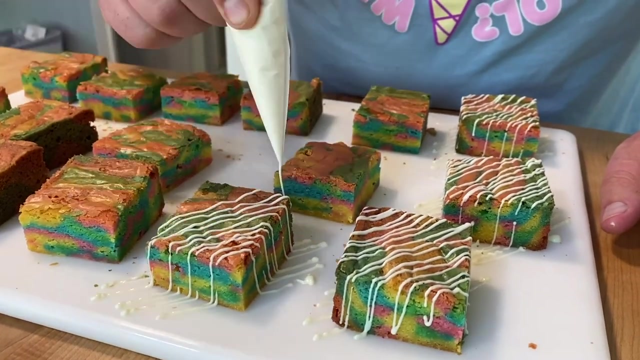 and you're going to cut a really small hole, really small, tiny little hole. Now let's decorate these guys. You see I'm going past the brownie. right, You want to go past the edge of the brownie. That's going to make it look professional. All right, finishing touch, Let's get a little glitter.